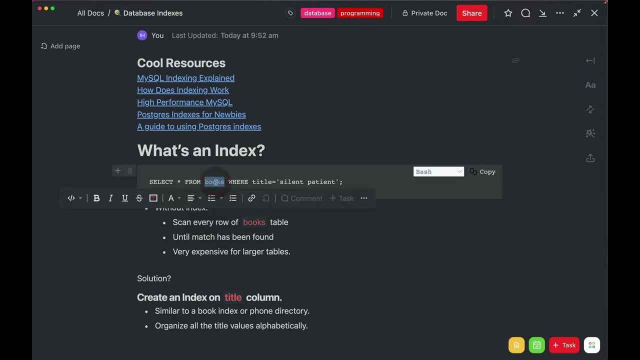 All right. so let's say we have a relational database and a table in it called books. This table contains all the books in our library. So we have a query over here. It's a very simple query. We're essentially looking at our books. 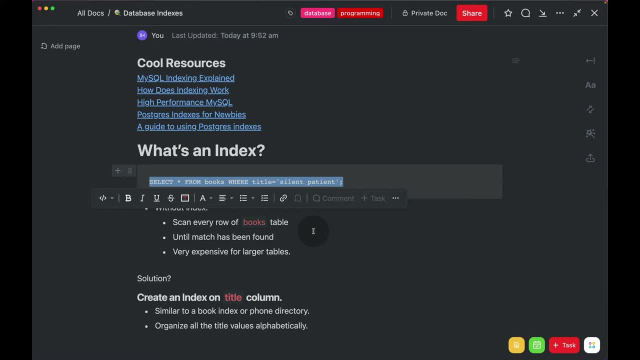 table and selecting the row with title set to silent patient. In a world where we do not have an index, the database is going to scan every row of the books table until a match has been found, Right. so if we have a million books in our table, 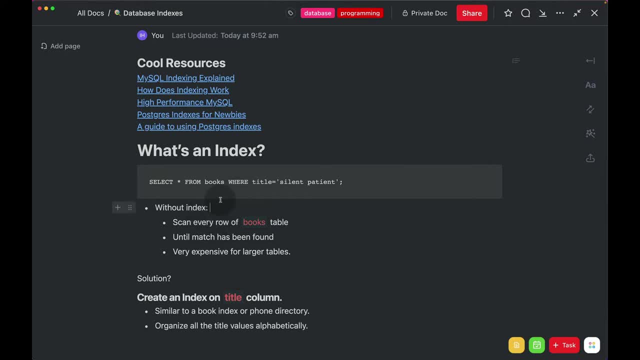 the database is going to scan every row of the books table until a match has been found. The database is going to go and scan all the million rows until it finds a book with the title silent patient. For a small table this can work just fine, But for larger tables 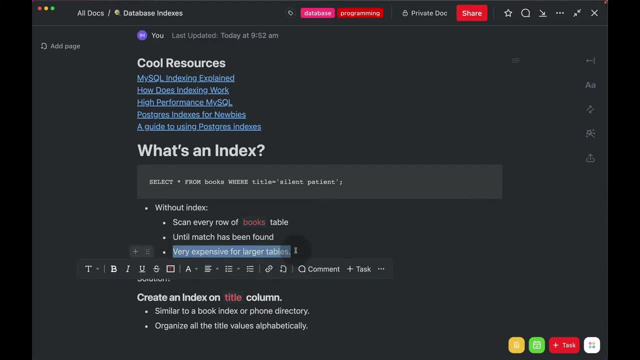 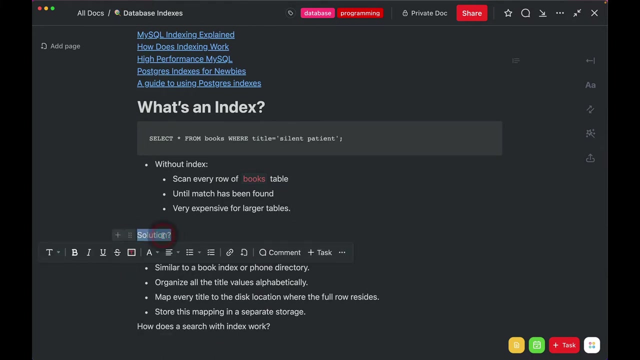 this can be very expensive. So if you have tables that have a few thousand rows or a few hundred thousand rows, doing a full scan of the whole table to find one row can get very expensive. Now what's the solution? So we of course don't want to scan all the rows, given it's going to. 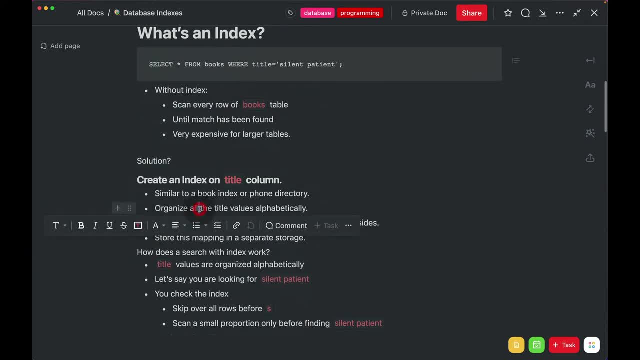 take longer. So the solution is going to be to create an index on the title column right. So we have multiple columns in our table, But we know that in this query we are searching the table by the column title, So we can go ahead and create an index on the title column. 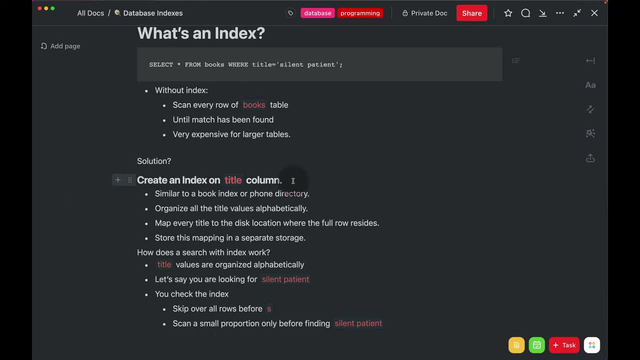 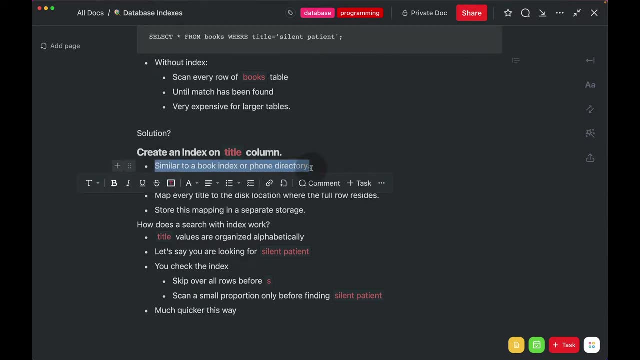 Now let's talk about what does this actually mean? When I say creating an index, what does it mean? So an index is similar to a book index or a phone directory, If you remember, in a phone directory, if you are looking for anyone's phone number, 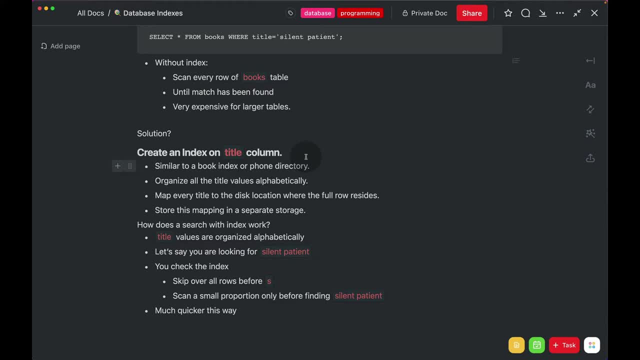 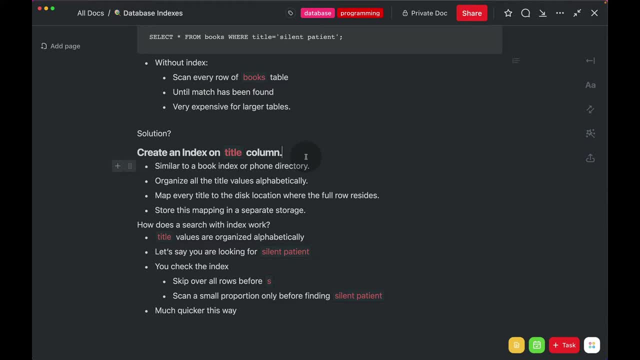 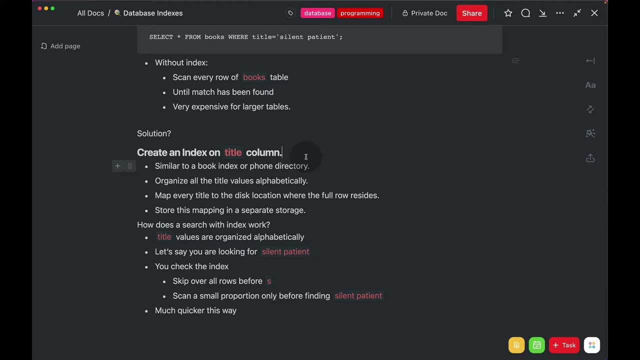 And then, once you find the contacts that are starting with M, you're going to start looking for max. So a database index is very similar. when you create an index on the title column, under the text box, the title column, what the database is going to do is organize all the title values alphabetically. 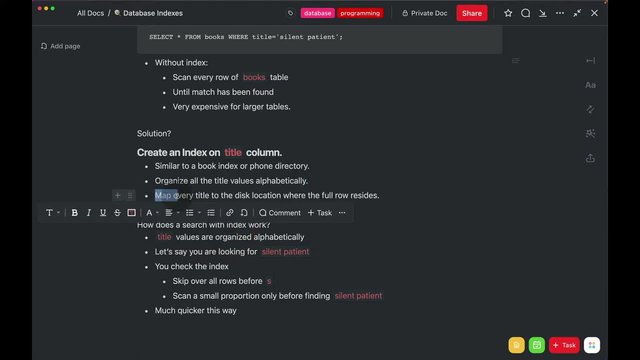 okay, and then it's going to map every title to the disk location where the full row resides and it's going to store this mapping in a separate storage. so what's essentially happening is, when you're creating an index on the title column, your database looks at all the different title values. 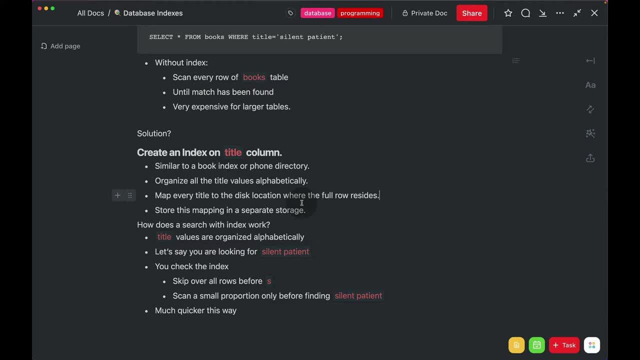 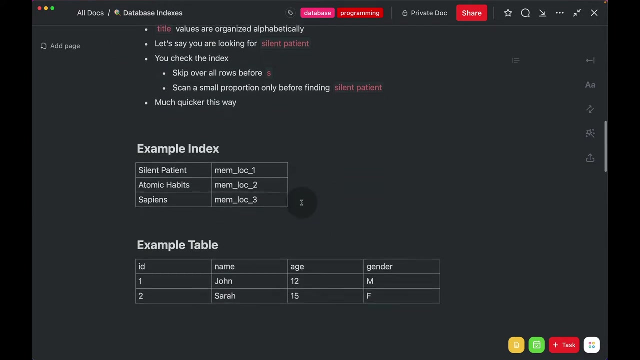 that are there in your database. it organizes them or sorts them alphabetically and then for every title value it creates a pointer to the disk location where the full row actually exists, and this whole mapping, or this whole index, is being stored in a separate storage. okay, so if we skip around a bit and look at this example index, the data structure that 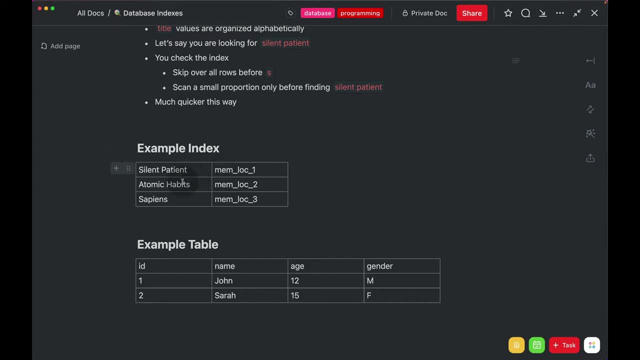 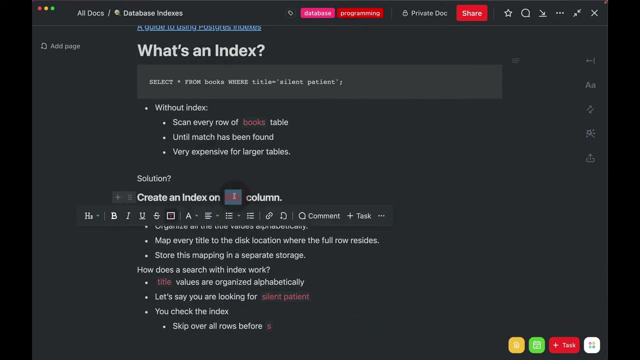 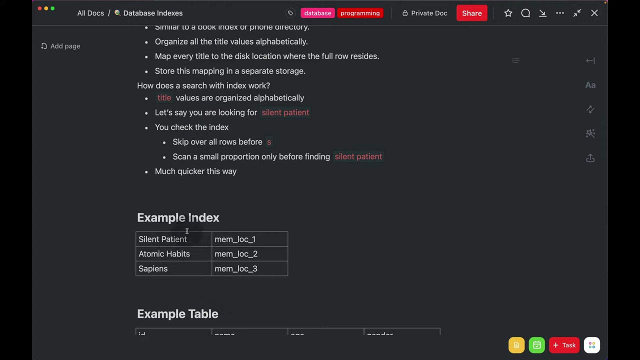 the database is creating to maintain the index is very similar to the table you see here. as i talked about, we are creating the index on the title column. so this is how your uh database is actually gonna actually gonna create the index. so i'm gonna create this in. 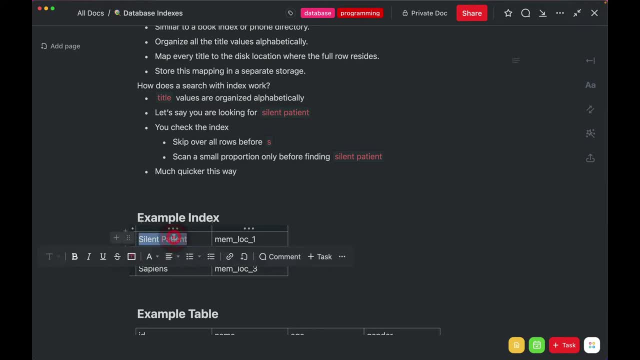 an alphabetical order to make more sense of it. so let's say we have atomic habits and then we have silent patient. okay, so you can see we have three rows over here and it's alphabetically ordered. for every row, so for every title, we have the memory location. so this is the memory location. 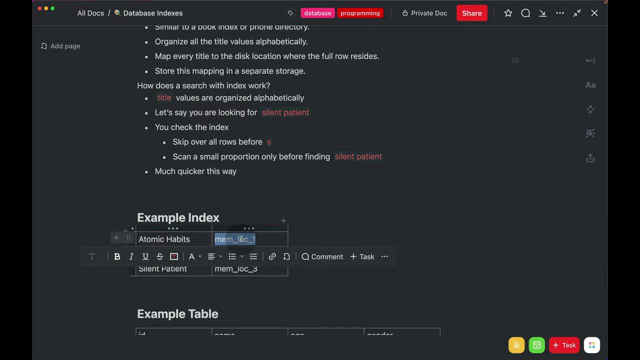 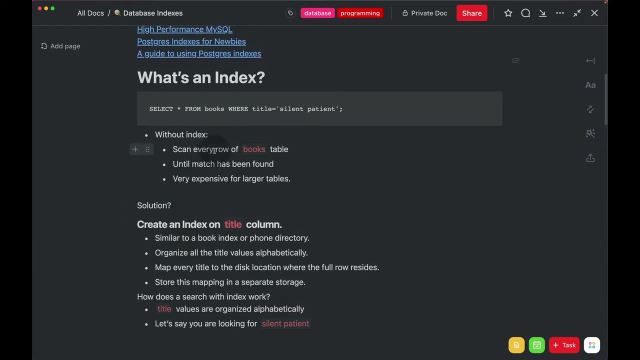 of the row and disk. right, so this is the memory location or disk location, whatever you want to call it, but essentially this is a pointer for a row that has the title atomic habits. okay, so this way, when you want to find a row with the title set to silent patient instead of 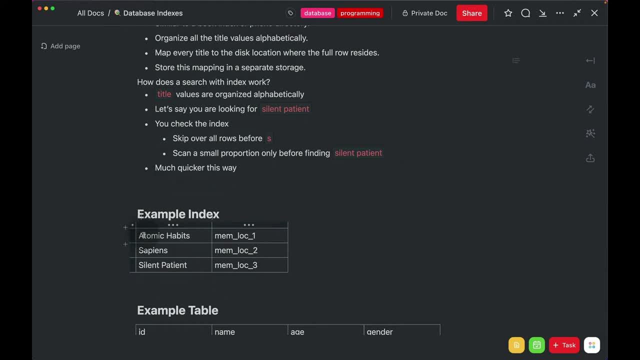 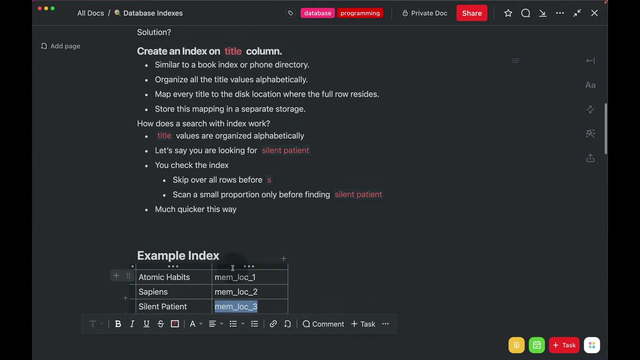 scanning all of it. you can go to the index, you can go to all the, you can go to the location where the entries are starting with s, and then you can go to silent patient, find the memory location and then actually go to the disk and fetch the row for a silent patient. okay, so how does this search? 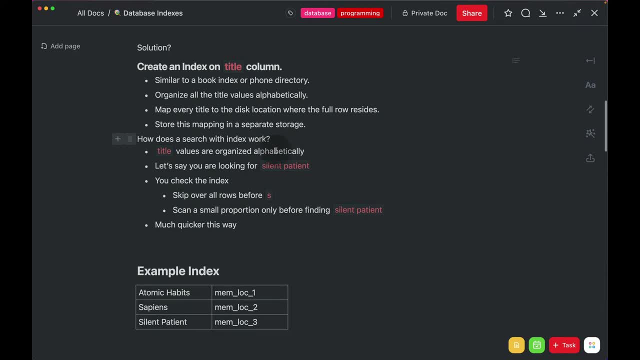 how does the search with index work? it's exactly how i explained. the title values in your index are organized alphabetically. let's say you're looking for silent patient. you check the index. you skip over all the rows before s. so in this case you skip over atomic habits. 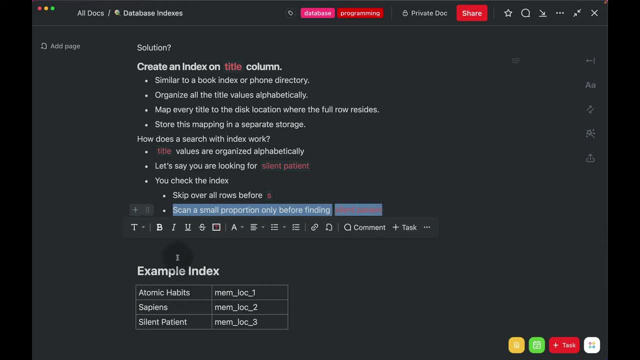 you scan a small proportion before finding silent patient. so if you're looking only at the first letter, you skip atomic habits. you're only looking at the first letter, so you skip the atomic habits. bips, you go to sapiens. so this is an entry with s, and then you start scanning sequentially. 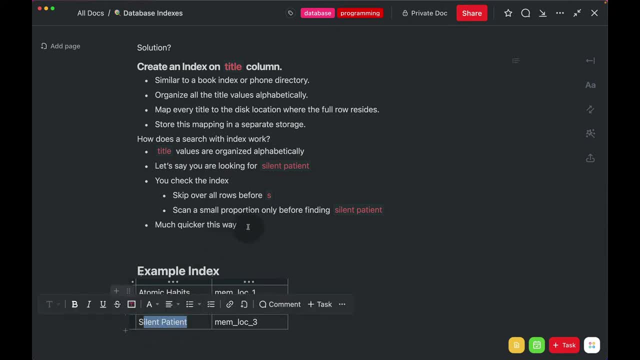 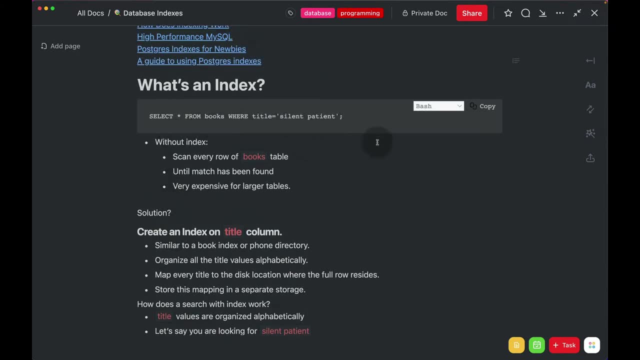 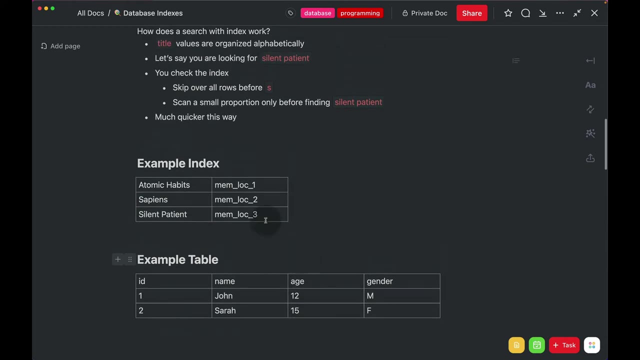 until you hit silent patient. okay. so this is much quicker to do it this way rather than do a full table scan for every single book. on the end the table: okay. so now we have an idea how the index looks like. let's talk about a different table now, okay. 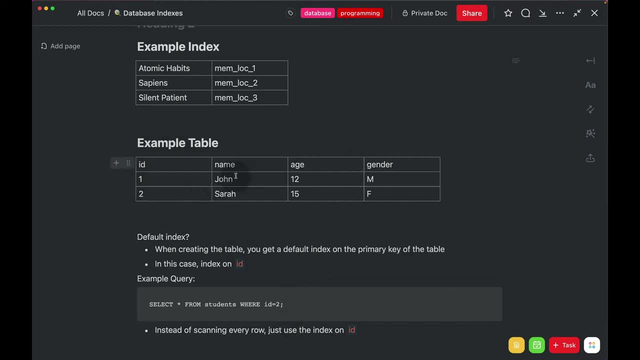 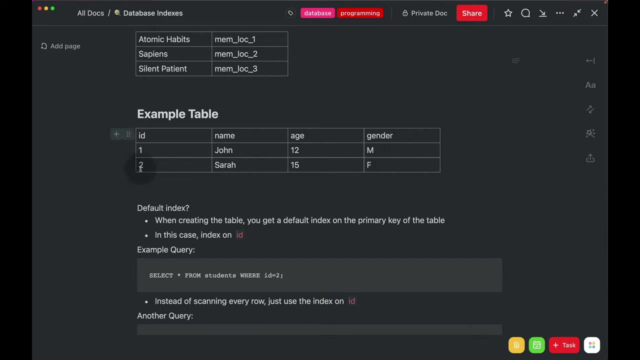 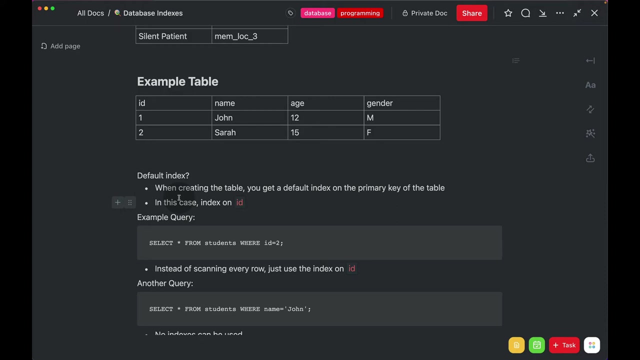 let's say we have a table with four columns: id name, age and gender. you can see that we have id one name, john, age 12, gender, male, and then we have two- sarah, 15 and female. by default most database engines- they are gonna create a table with four columns and then they're gonna create a table with: 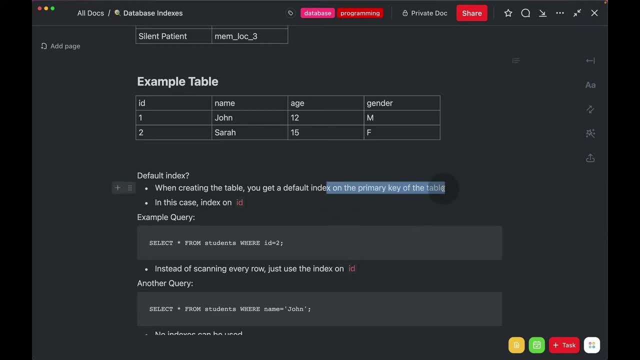 two columns and then they're gonna create a table with four columns and then they're gonna create a table with create an index for you based on the primary key of the table. So in this case, our ID column is the primary key, So the table is already going to create an index for you for that ID column. 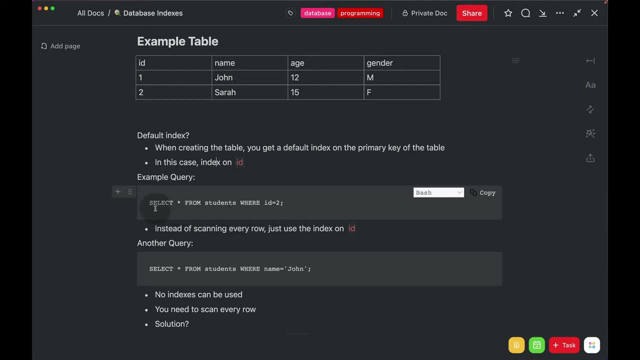 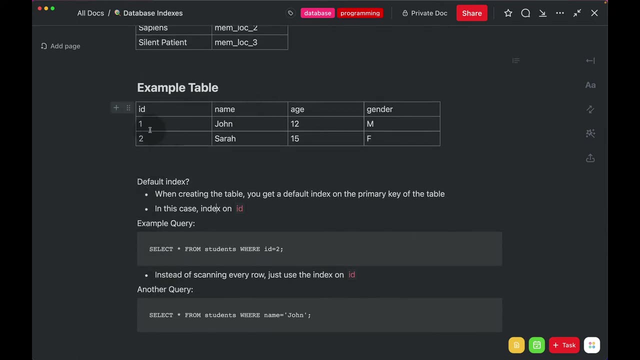 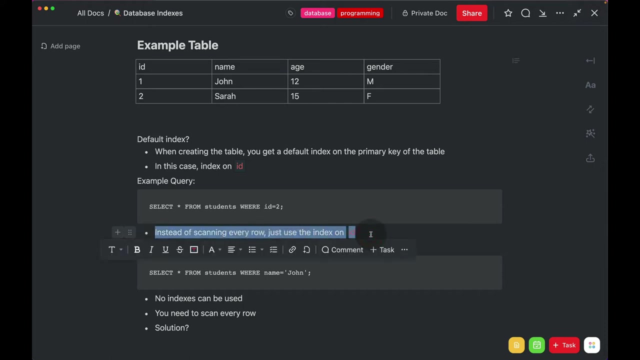 Now, if you have a query, example would be select star from students where ID equals two. So we're calling this table students and we want to find the row where ID is set to two. Now your table, instead of scanning every single row until it finds one with ID equals two. 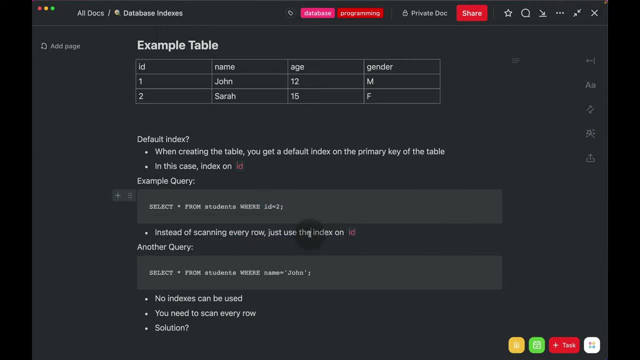 it's just going to use the index on ID and very quickly give you the row. This is something you get by default most database engines. they are already going to create an index on the primary key, which, in this case, is going to be the ID column. Now let's look at another query. So 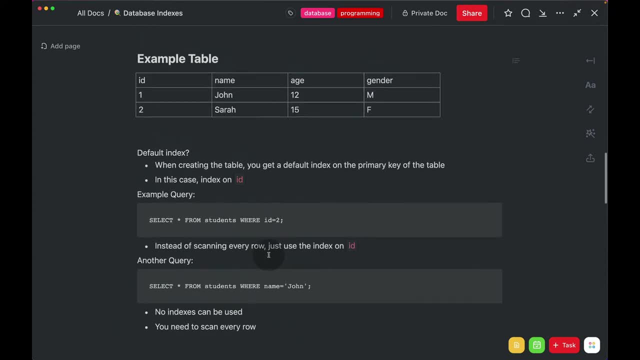 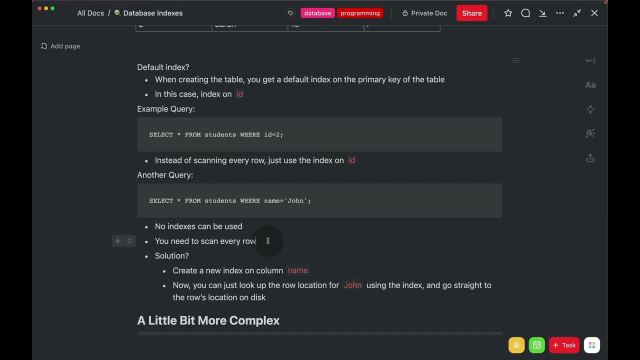 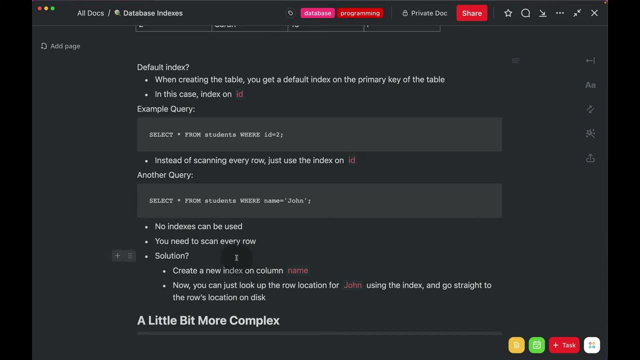 again, this can get very expensive for large tables, So a solution would be to create a new index on the column called name. Now, when you execute the same query, you can just look up the row location for John Using the index and go straight to the rows location on disk. So I am switching between. 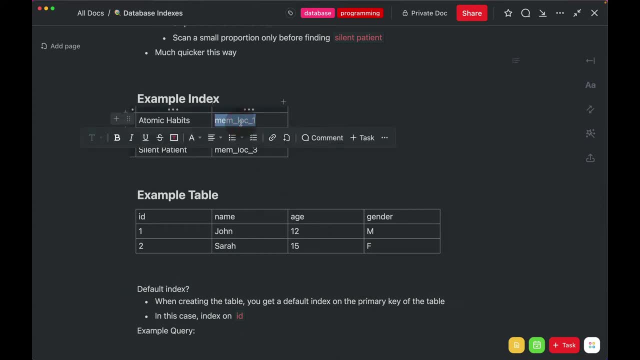 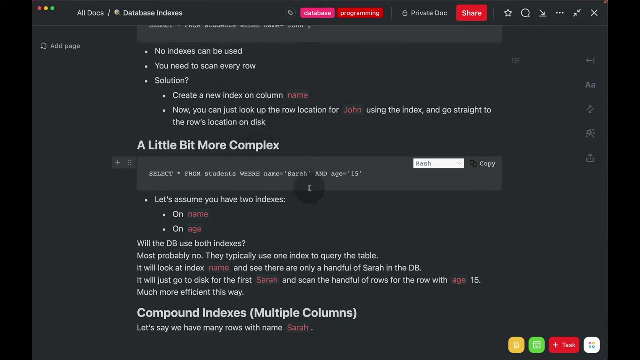 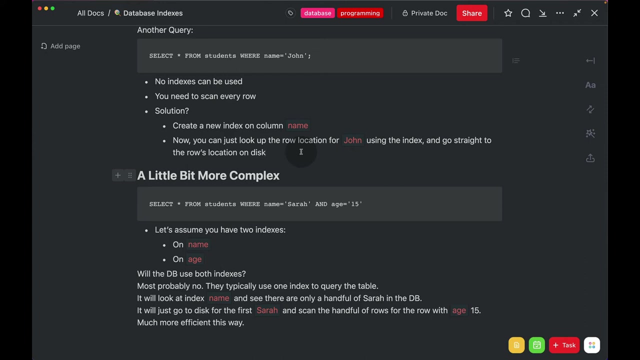 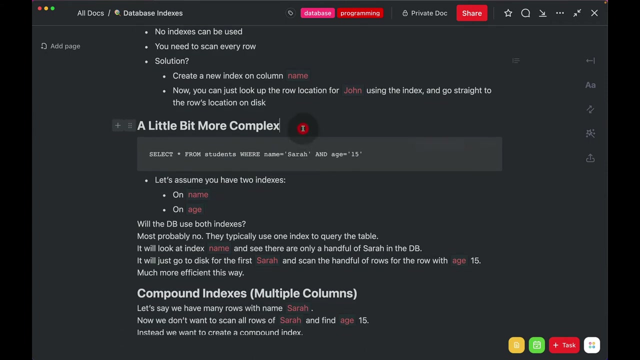 memory location and disk location. Essentially, this is a pointer to the location of the row. Okay, so in the most basic terms, that's how an index works. It makes lookup queries very easy if you are indexing the correct column. So now let's let's talk about a little bit more complex use cases. Let's say now your query is as: 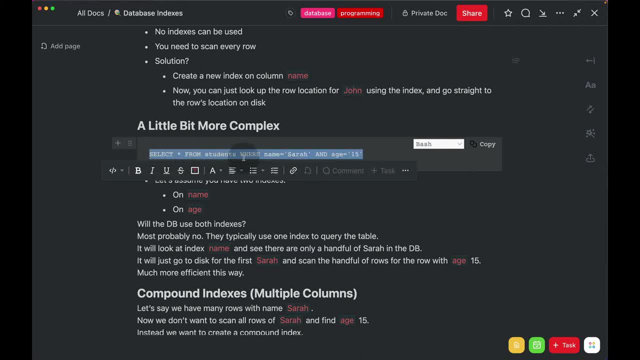 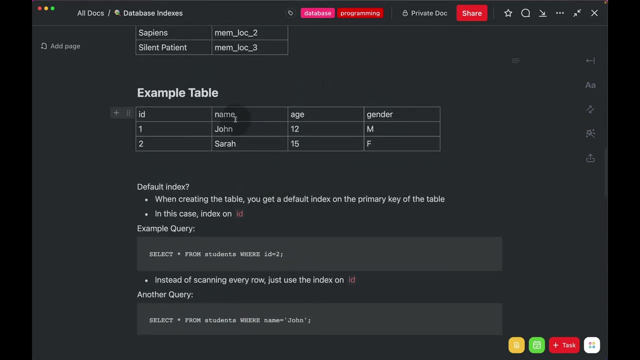 such you have select star from students where name equals Sarah and age equals 15.. Let's say you have two indexes in your table. One index is on age, another index is on name. Okay, so we have two rows, name and age, and we have two separate. 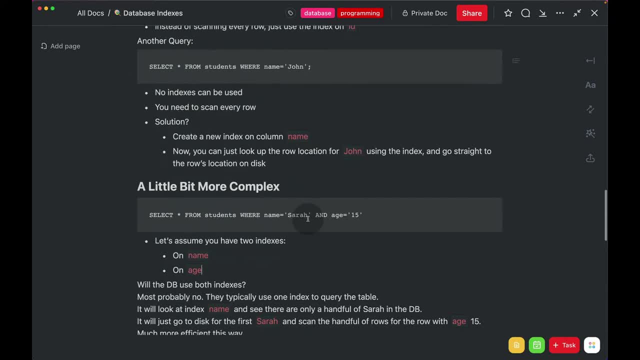 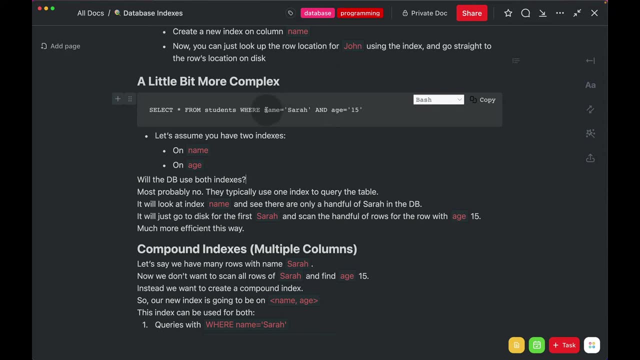 on both of these Okay. So the question is now that in your where clause you have: name equals Sarah and age equals to 15, so you are querying by two columns at the same time. will the database use both of your indexes at once? The answer to that is most probably no. Typically databases. 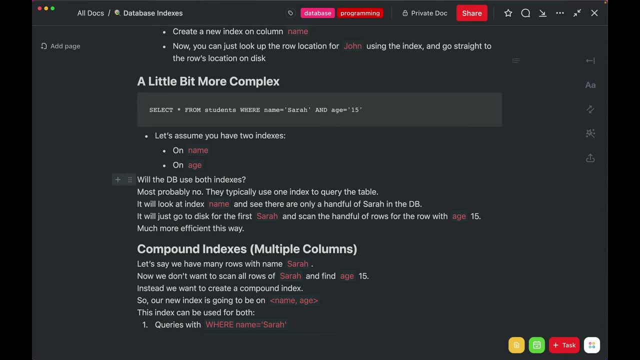 use only one index to query the table, just for performance reasons. So in this case, your database- it's going to look at the index name, because that's the first thing you're querying by, And it's going to see that there's only one row in the table with the name equals Sarah. 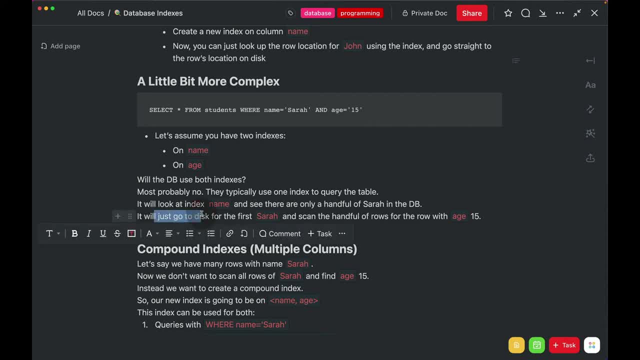 In that case it can just directly go to disk after it talked to the one index and get the row with the age. Okay, Now you might ask what if we have multiple rows of Sarah, So maybe Sarah age 15, and then we have Sarah age 20,, Sarah age 25,, multiple of them? What your database can do is: 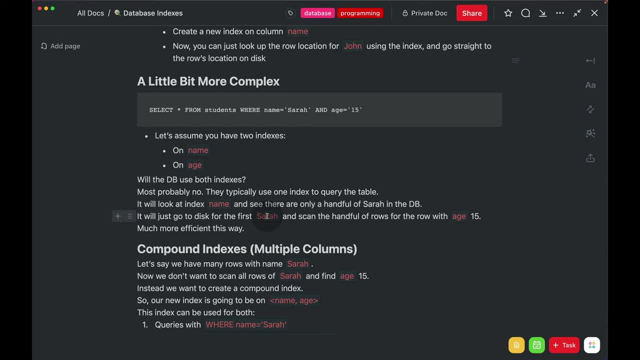 go to the first Sarah and then do a sequential scan until it finds a Sarah whose age is 15.. It's much more efficient this way than consulting two separate indexes And database. for a lot of cases, even if you have two indexes, it's going to end up using one to get better. 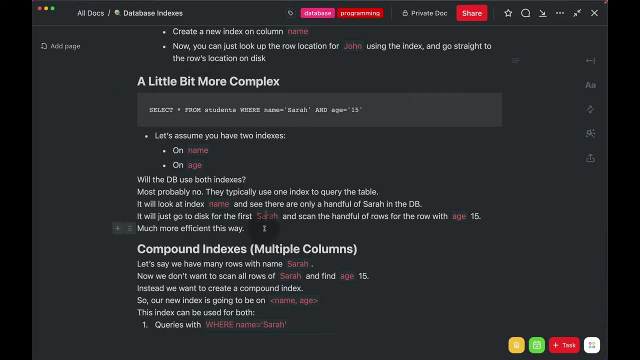 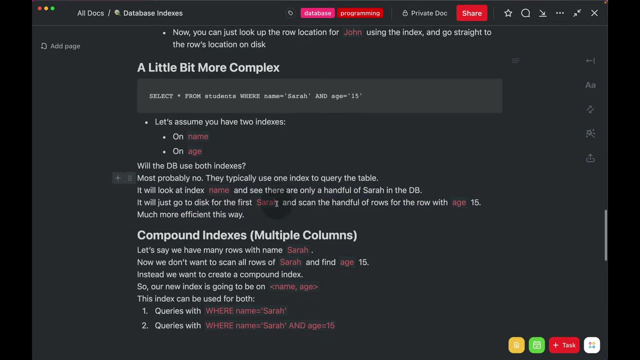 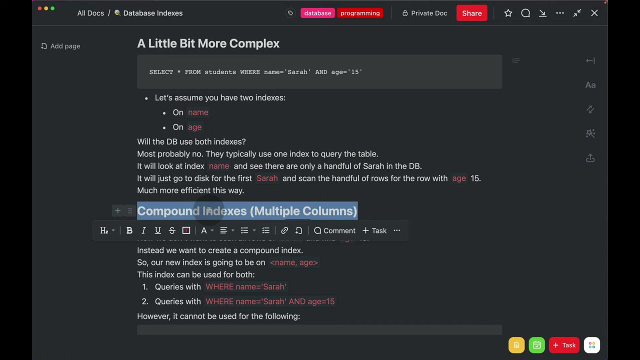 performance. So that's how databases can decide against using multiple indexes at once. However, you can have something like a compound index, right? Compound index is very different from having separate indexes for individual tables. For compound index, you can have one index based on multiple columns. In this case, let's say you are creating a compound. 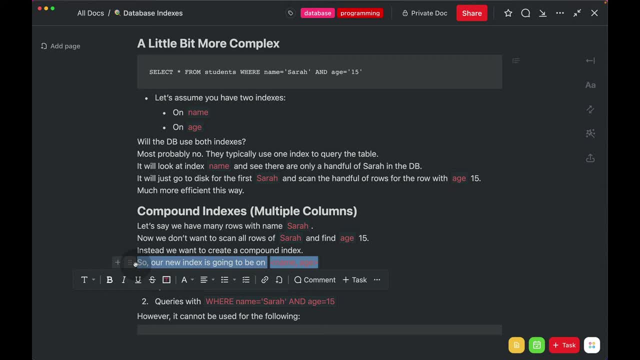 index on the combination of name and age, And we're going to make the assumption that in your database or in your table, you have many rows where the name is Sarah, So you have many Sarahs in your table. Now let's talk about the same query You want to find. 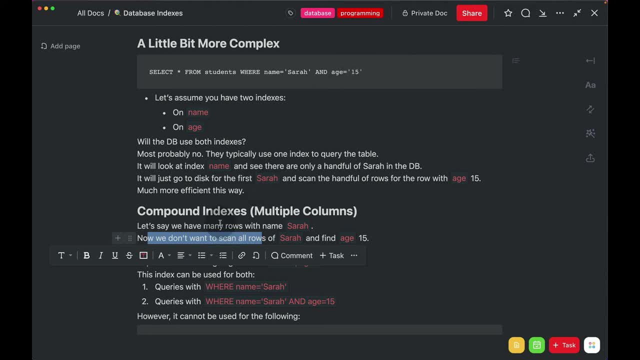 Sarah whose age is 15.. Unlike the last, unlike the last time, where we knew that there were only handful of Sarah in our database table, Now we have many different Sarah. So, instead of using only the name index, so only this index, we are going to be using our compound index, which is going to: 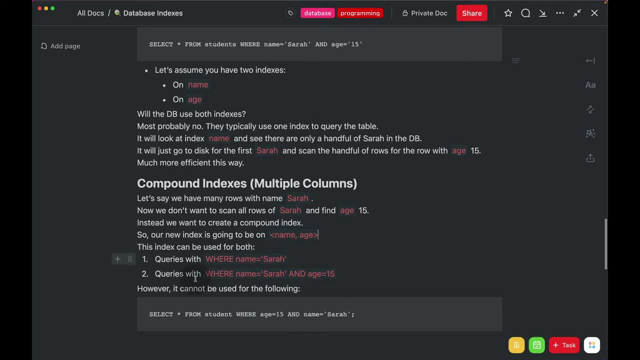 be name and age. Okay, And now, instead of going to the first Sarah and sequentially scanning all the rows until you find Sarah with age 15, we are going to use the index to find all Sarahs whose age are 15 and then go and fetch them from. 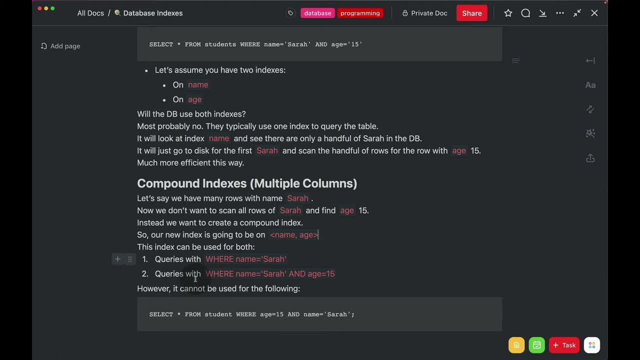 the disk. Okay, So this way we are avoiding doing a sequential scan on all the Sarahs in our database. Instead, we know exactly where Sarah, whose age is 15, resides in our database. We consult the index, find that row and then bring it back to the user. 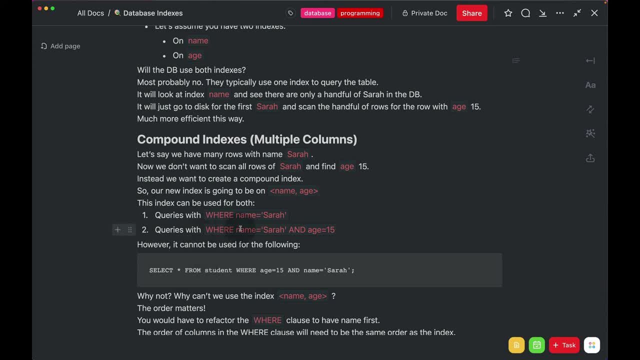 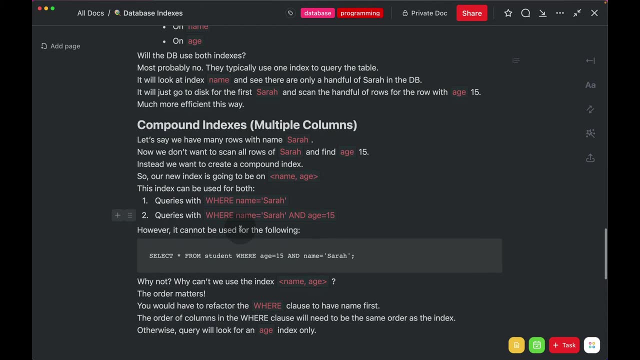 Now, one cool thing about compound indexes: it can be used both as a compound index and a single index. To give you an idea, let's say if your query was something like this, where name equals Sarah, so you're only querying by name. 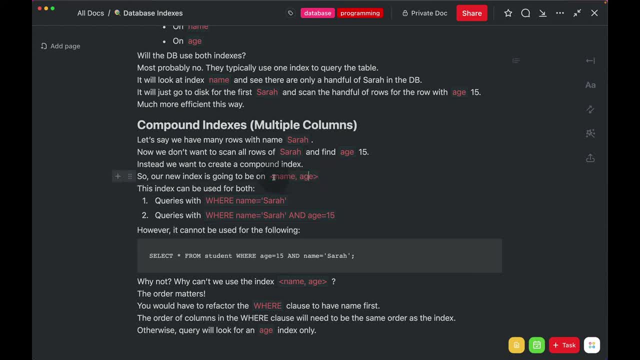 You can still use the compound index, even though your index is set on the combination of name and age. For queries where you're doing name equals Sarah, you can still use the index And, of course, if your query is something like name equals Sarah and age equals 15,. this is the example we talked about before. we can go ahead and use the compound index, because the index is organized by name and age. 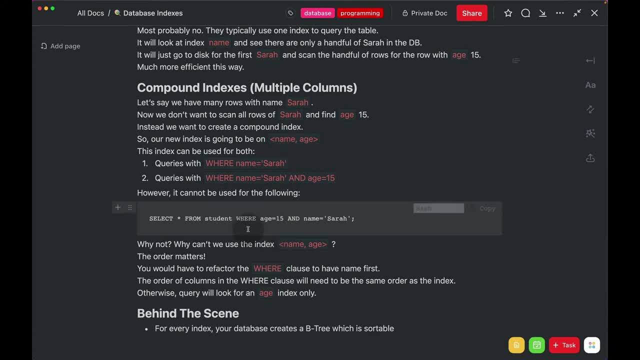 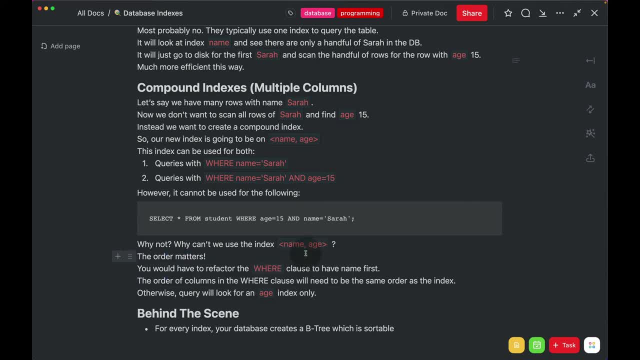 have name at first, age second. Because the orders are different, you cannot use the compound index or this compound index for the query above. You would have to refactor the where clause to have name first. So you would have to do where name equals Sarah and age equals 15.. The order of columns in the where clause will need to be the same order as your compound index. 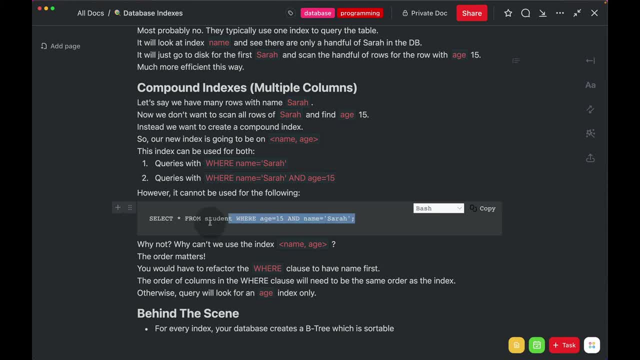 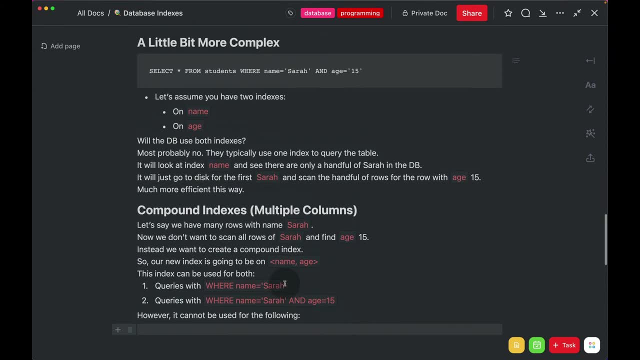 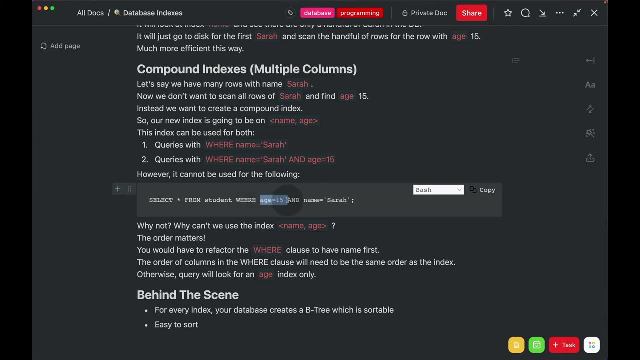 Otherwise, if you keep this query as is, your database will look for an index- age, right. So remember we did have an index on age, Your database engine, it's going to look at the first column of the where clause, which is age, and then look for an index that is either on age or starts with age. Okay, so that is a subtle difference between. 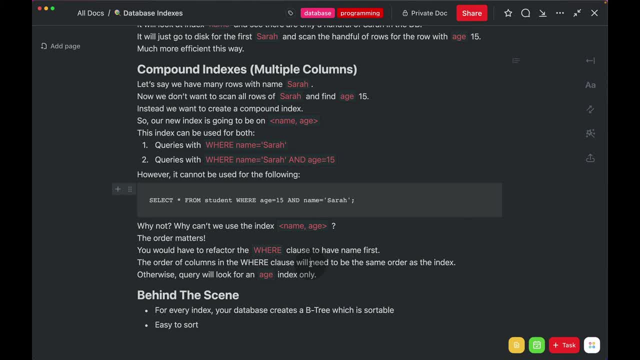 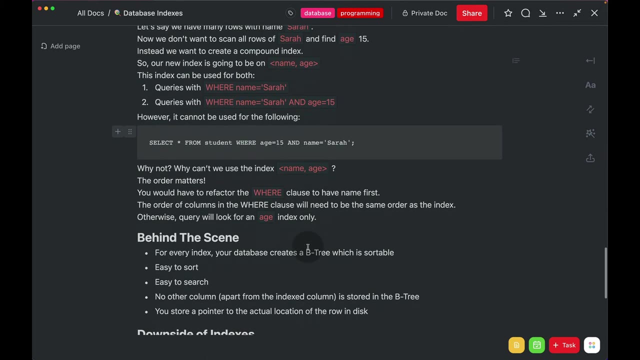 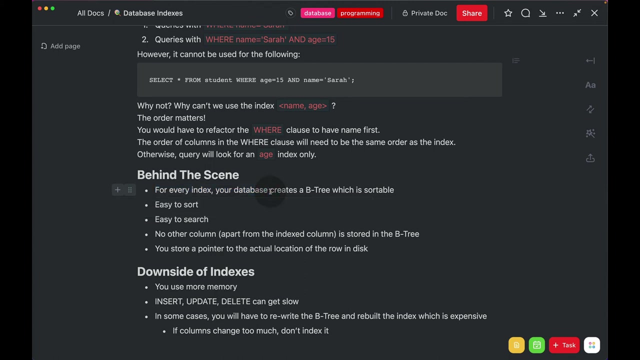 different times, that the database engine can either decide against or for using an index, And you want to keep in mind that the order over here matters when it comes to whether the database is going to use an index or not. Okay, so now let's talk about a little bit behind the scene and what actually happens when you create an index. For every index you create, your database creates a B tree, which is a database. 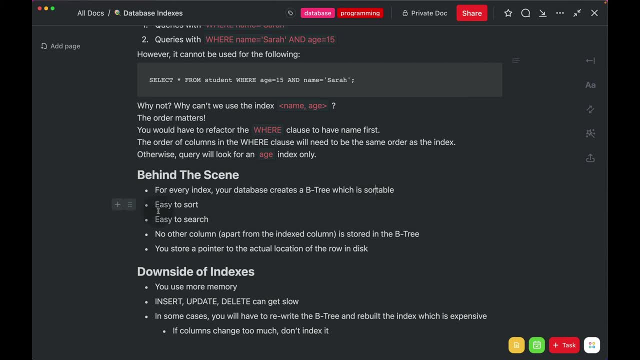 data structure which is very easily sortable. As mentioned, B trees are easily sortable And it's also very easy to search for something. When I say that the database, the database, is creating a B tree for every new index, it is not actually storing your whole row in the B tree. Instead, what? when you create an index in the B tree, the database is inserting the column of the index. 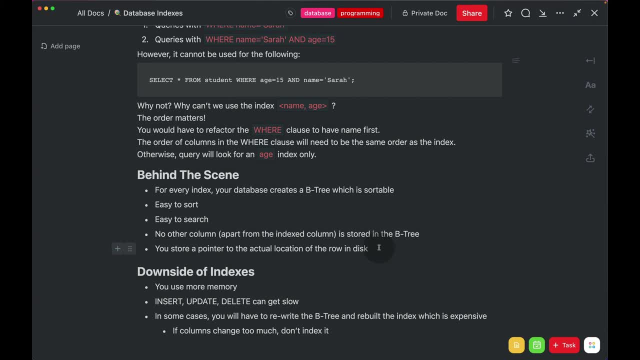 of the index. So if you're indexing on the column title or on the column age in your B tree, the only piece of data that's going to be there is this column value. So, whether the age value or the title value, With that value in every node of the B tree you are going to store a pointer to the actual location of the row and disk. So let's say, if you have age equals 15.. Right now, your, your, 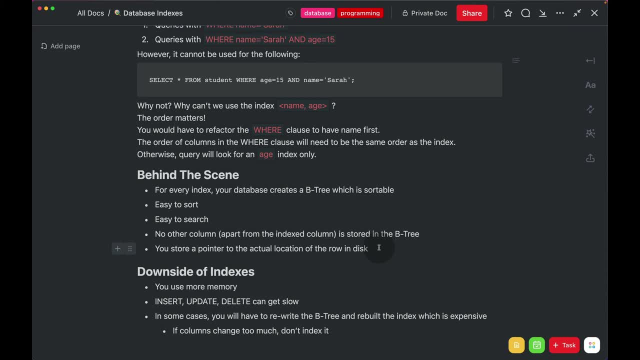 database or your B tree. it's going to store that 15, that value, 15.. And then a pointer to the row where this, where the row, where the full row with age 15 is okay. That way, even though you can create multiple indexes, your space, the amount of space you're using, it's not going to be exactly the same space as the database. it's going to be very little, because you're storing the value and the pointer only. 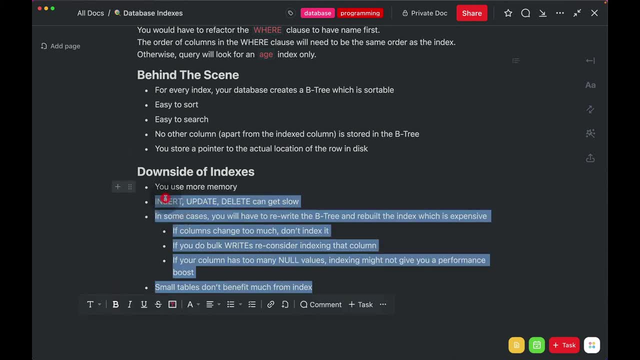 Okay, so we're going to wrap it up by talking about some of the downsides of indexes, because it might look like the only solution to optimize your queries is going to be adding newer and newer indexes. However, that's not really a good practice And you want to be mindful about when adding any new indexes. The first thing is you do use memory when creating index. Every time you create an index in the back end, you are creating a B tree. 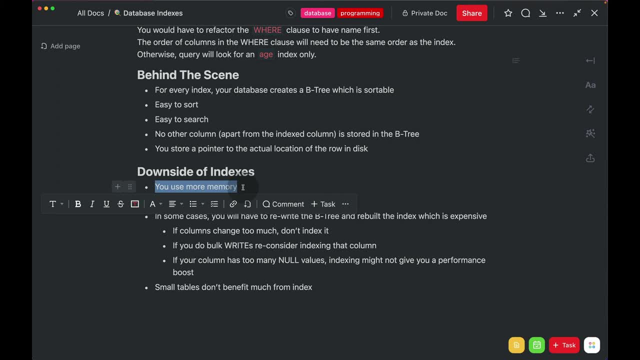 with the value of the index and the value of the index column and the memory locations associated with it. So the more indexes you create, the more B trees need to be built, So more memory is being consumed. Also, every single time you create an index, or the more indexes you have, your insert, update and delete operations can get very slow. This is because whenever you are 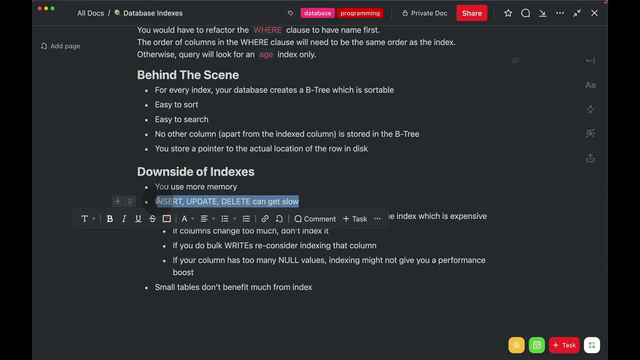 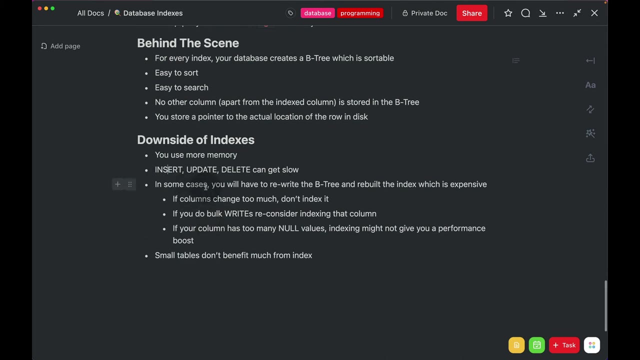 inserting new data, updating old data or deleting data, your index needs to be updated too. So the more data you write or update, the more your indexes need to change. Hence the operation can get slower and slower. As talked about, in some cases you will have to rewrite the whole B tree and rebuild the whole index, which is expensive. So not only do you have to update the index, but you also have to update the whole B tree. 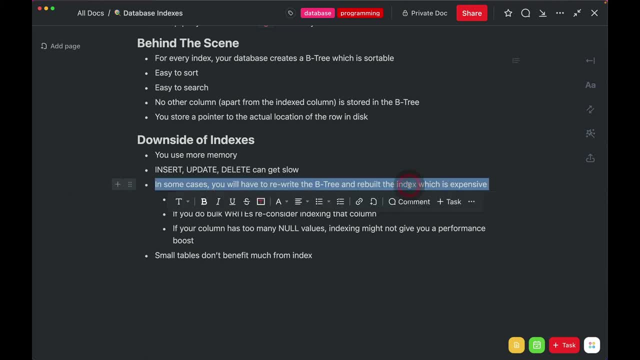 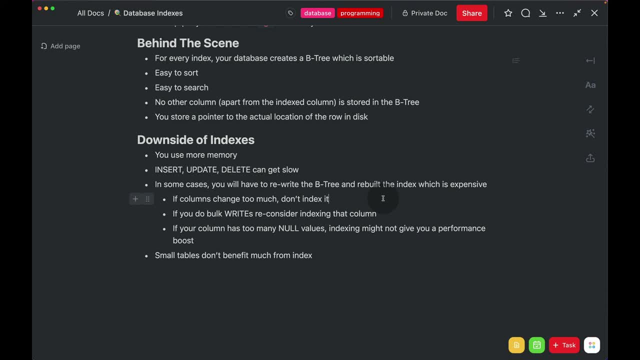 So if you have a table where you have a certain column that keeps changing depending on your application needs, don't index that column, Because every single time you update the values in that column, your database will have to go tweak or even rebuild the index, which can be very expensive. 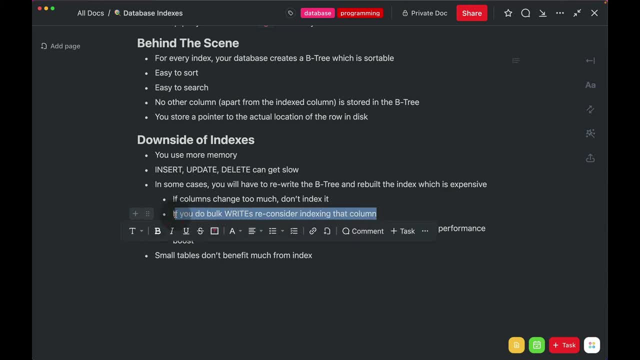 So if you have a use case where you have some kind of a batch job that does a bulk write- so let's say it writes a few hundred thousand or a few million rows at once- make sure you don't have too many indexes, because every time you are doing this bulk operation, if you have too many indexes, all of them would need to be updated, which can make the whole write process very, very slow.